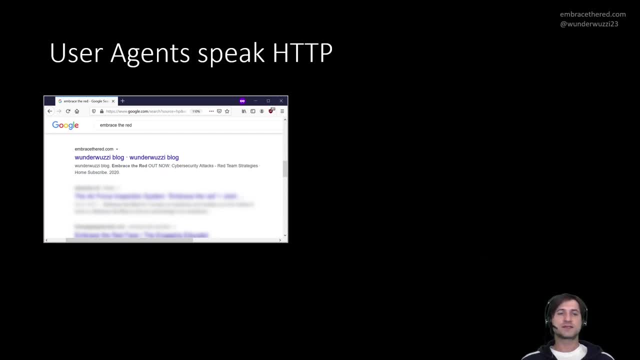 For us, user agents, like initially, just think about a user agent being the browser. Like all the RFC documents, the request for comments, Like the specifications of the World Wide Web, they always refer to the browser as a user agent And basically a user agent is any application that sort of acts on the user's behalf. 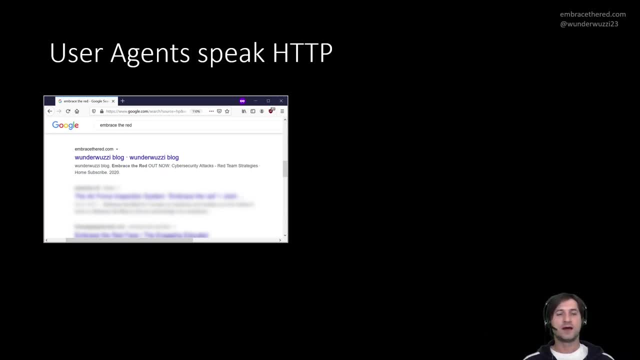 And the most common ones we use are browsers- right, And you might be familiar with Firefox, Chrome, right. Those are user agents and they speak the HTTP protocol. HTTP stands for hypertext transfer protocol, And that is sort of the language on how the code is rendered. 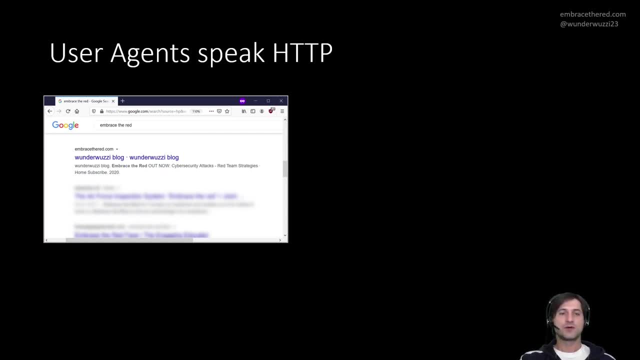 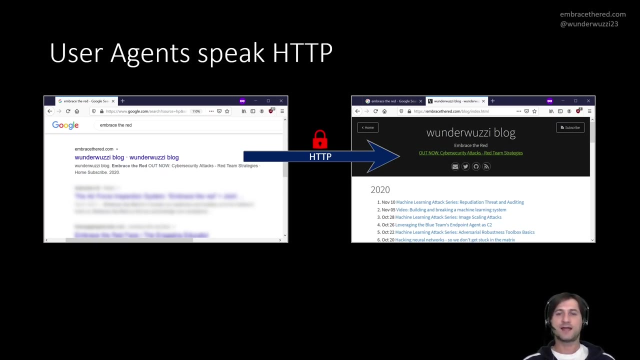 How communication happens in the World Wide Web. So think about this: You have your browser open, right? You do a Google search and then you click a link in the browser And that link- now this click- creates an HTTP request that takes you to this other website that you clicked on, right. 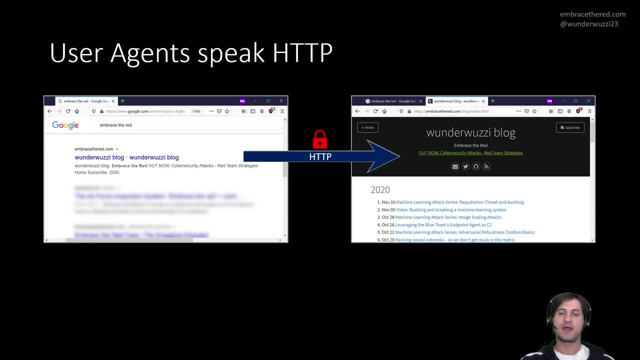 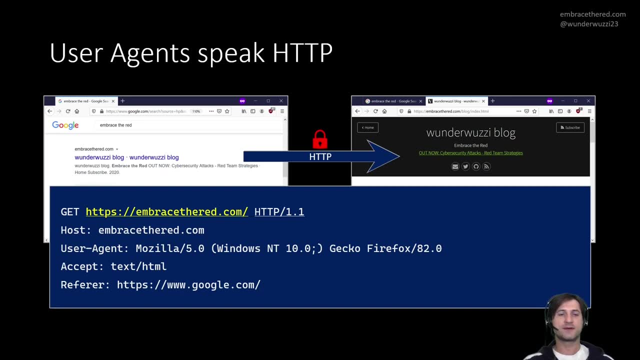 This is sort of this idea of hypertext transfer protocol and hyperlinking, And when this happens, right, The browser actually issues a HTTP request, a GET request, And that looks like the following: right, It has this GET, which is called the verb. 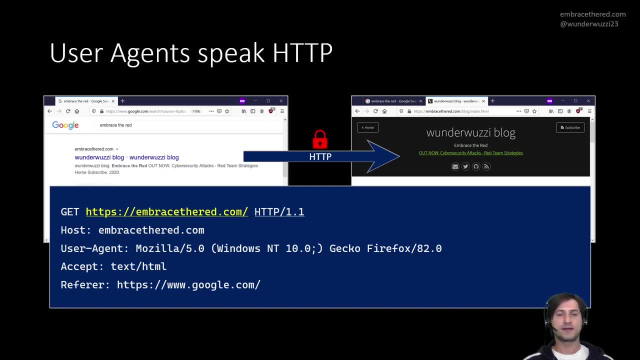 Then it has the destination, link or URL, The protocol that it is using, And then a set of HTTP request headers that sort of send additional information to the web server that it is communicating with. You can see here, for instance: right, It would send the user agent. 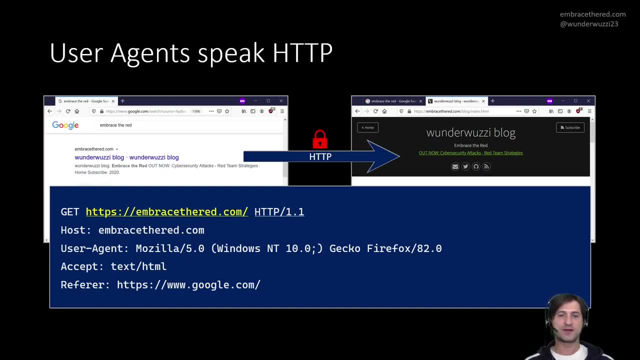 Which we just described. That is the browser. In this case, it's like Mozilla Firefox, right? It sends the version number And then it sends other important or interesting information as well, For instance, a referrer header Which tells the web server that you're visiting where you actually came from. 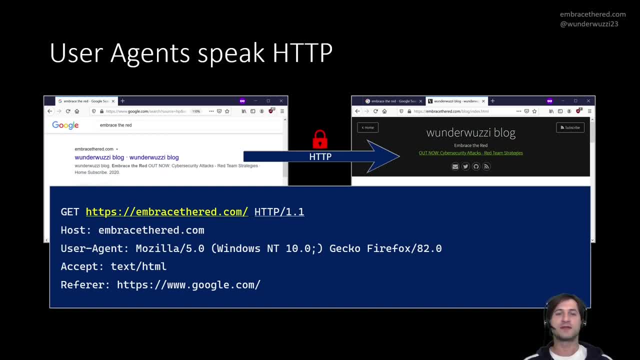 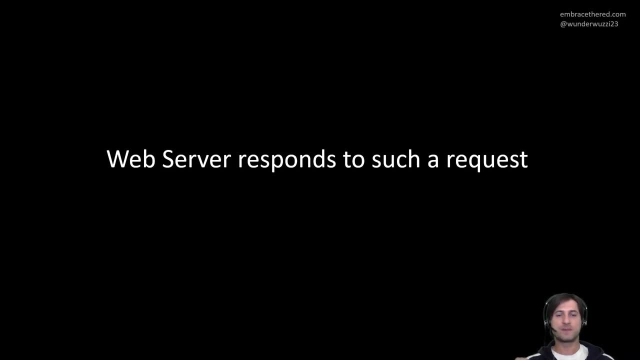 Like which site or which origin you came from in the web. So that's very interesting information that the web server can gather about you just clicking a link. So what is sort of then happening on the other side right? The web server now gets this request and the web server responds to it. 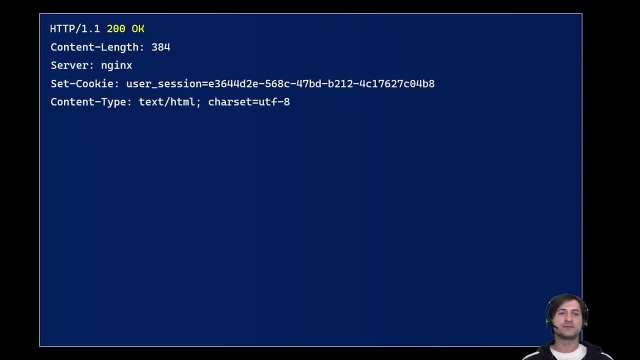 And the way a response looks like is the following: So it is again text-based, It sends back the version number And we call this on the top here the response headers, And in the very beginning you also have the status code that you can see here. 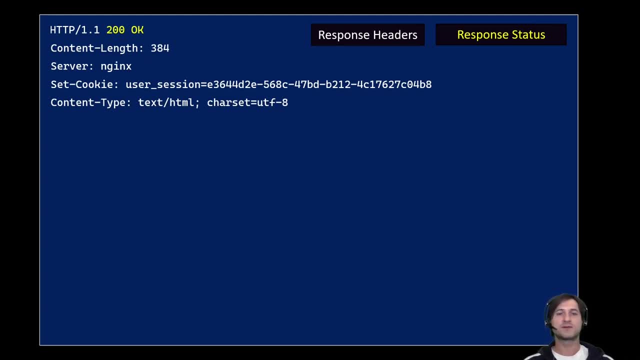 200. OK, That means that everything went well on the web server side, And it's going to send you now the response. It contains a link what kind of server version the web server is running. It might then contain additional response headers about setting a cookie. 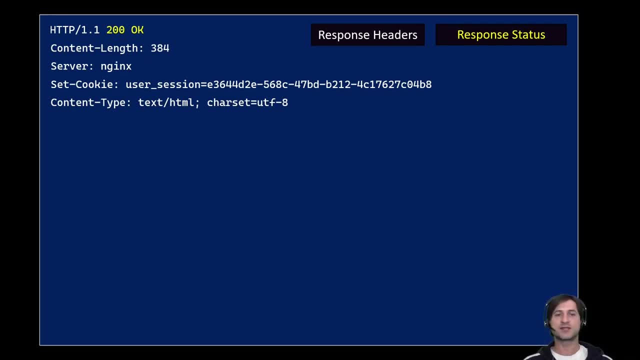 Which we'll talk a lot in more detail because that's very security sensitive And it's also important to understand the content type HTTP response header. So the content type talks about how the browser or the user agent should interpret the result in the body of this message. that we'll look at soon. 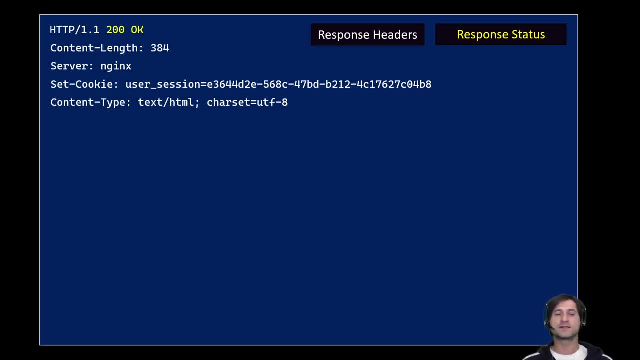 In this case, and it's very common that this is text, HTML, So it's hypertext markup language. But this could also be just JavaScript, or this could be a binary blob or an image, for instance. So in our case we have an HTML document. 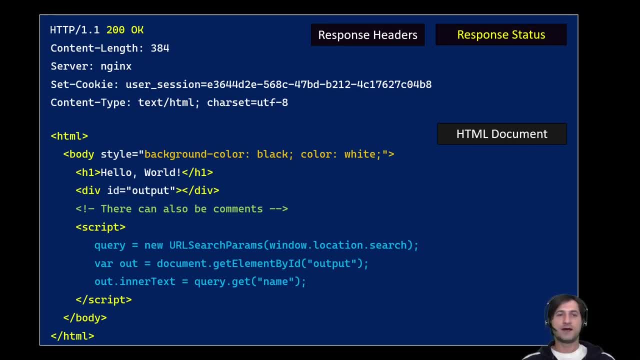 And this is sort of how response looks like. We have HTML, We have HTML elements in the document. I'm going to describe this a little bit better in the next slide as well, But sort of this is how an HTML document looks like. 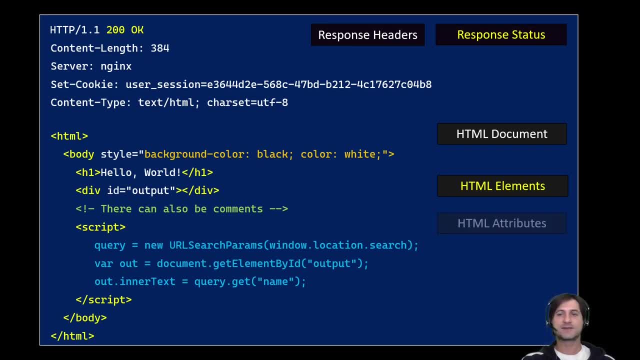 We have HTML elements, which is sort of the tags. We have attributes, which sort of further refine what an element looks like or what kind of attributes an element has, Like it might have an ID, a name, a style. Speaking of styles: 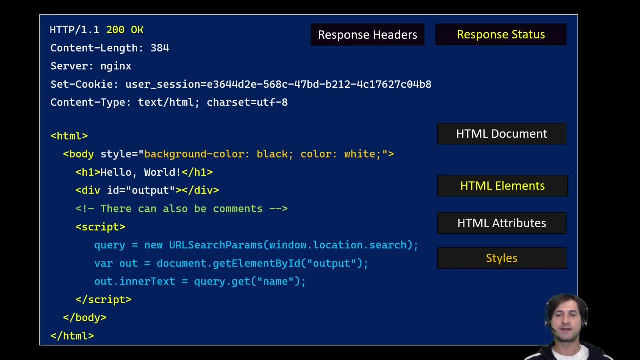 you might want to define the style on how this HTML element is actually rendered, what color it has, what transition behavior you might want to define. And then, very important also, is the code. So HTML documents can contain code, And this is sort of where, from the security point, it becomes very, very interesting. 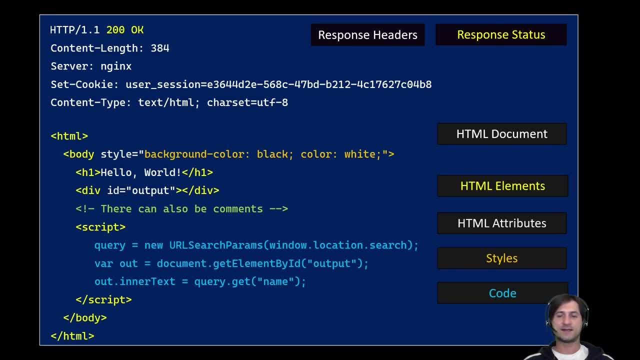 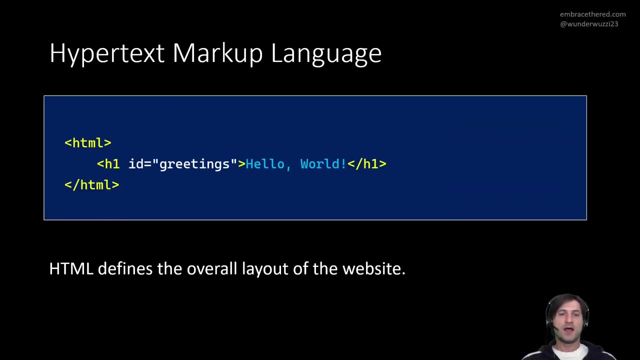 So I'm going to have another slide that talks much more about this code concept, And then also we're going to have dedicated sessions, for instance, about very common vulnerabilities that happen when you have something like code injection. But yeah, let's look a little bit more now into these very basics. 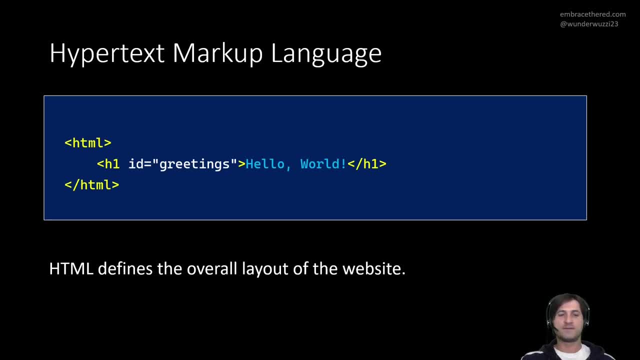 So you have the hypertext markup language. These are HTML tags, or HTML elements, right. Then you have attributes which sort of further refine the tags. we said these elements, And then you kind of might have string literals Which is sort of, in this case, hello world. 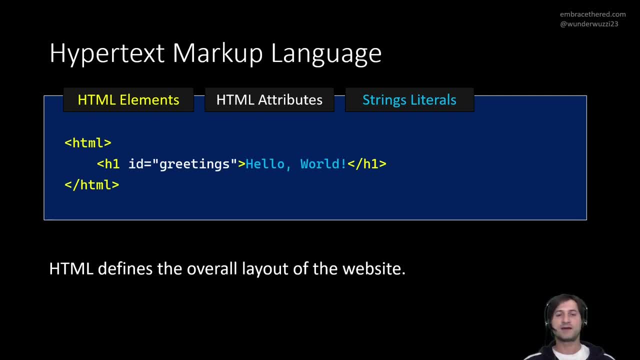 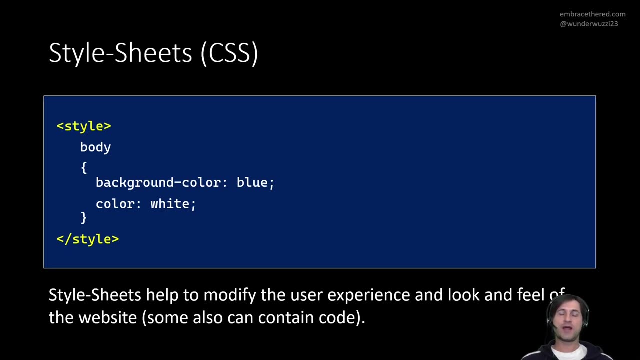 So this will print out kind of a large header that just says hello world. So that's sort of the overall idea of the markup language. And then we have style sheets which are basically describing how these elements should be rendered. In this case it would say: hey, the body element. 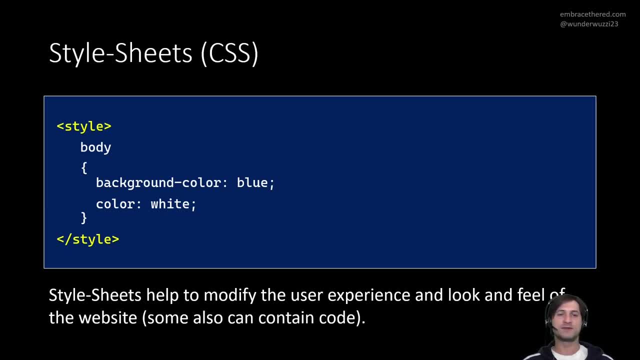 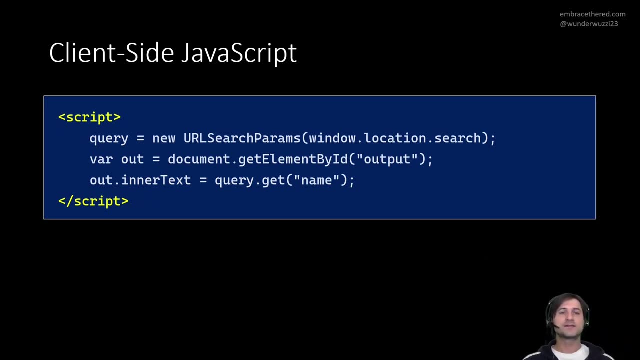 the body HTML element should be rendered right with a blue background and the fonts should all be white by default everywhere on the page. So this is sort of the kind of behavior you can drive with style sheets. And the third concept again, the JavaScript execution on the client site, right. 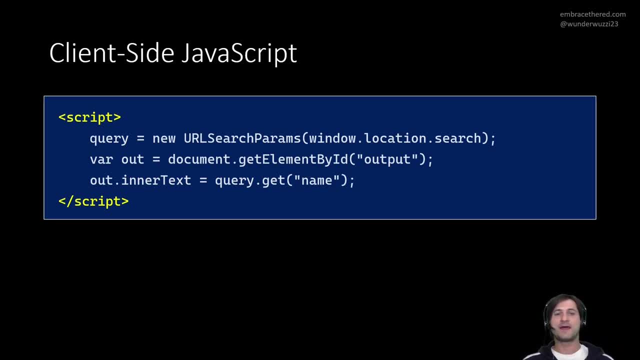 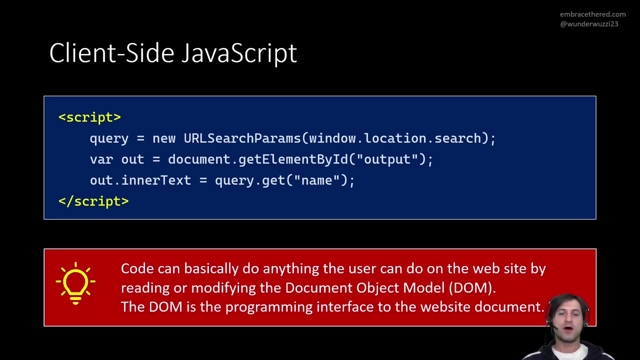 It starts with the script HTML element tag And then it actually is just arbitrary code that is then being run by the browser And it gets intact with the web page, And the way this interaction happens is by the document object model. So the DOM is basically this programming interface. 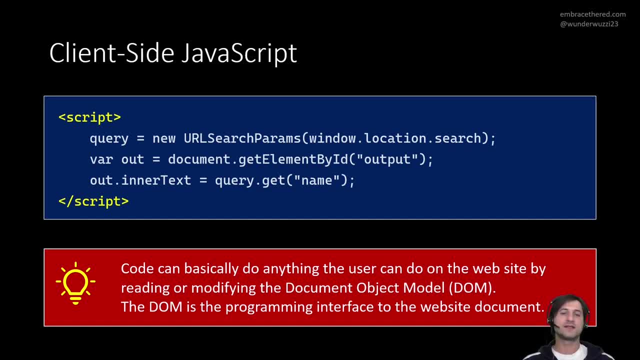 that JavaScript has to interact with the HTML document And then JavaScript can read from the document, It can update elements in the document, and so on. So this is sort of this idea of this document object model, And what is so important to understand is that 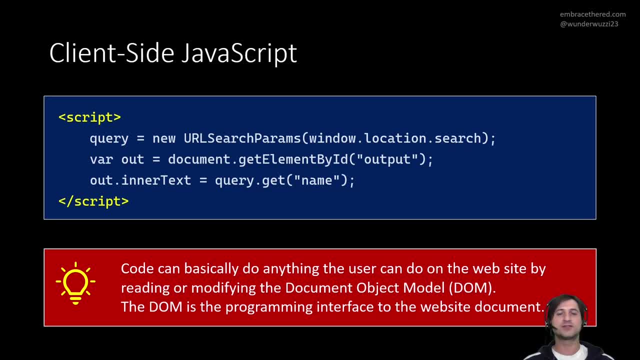 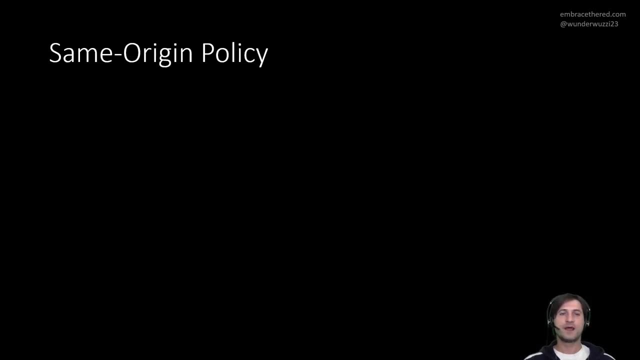 JavaScript can basically do everything that the user in front of the computer can do with this web application, And this is sort of important to grasp. So the code can modify, read any data from this particular web application, And you might have noticed that I said from this particular web application. 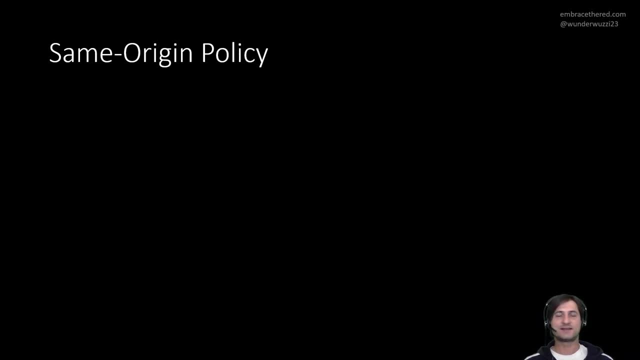 because to understand the security of the Internet, there's actually not a whole lot of security concepts, but there's a whole lot of security concepts, And this is sort of interesting when it comes to the web, The one thing that sort of everything hangs upon. 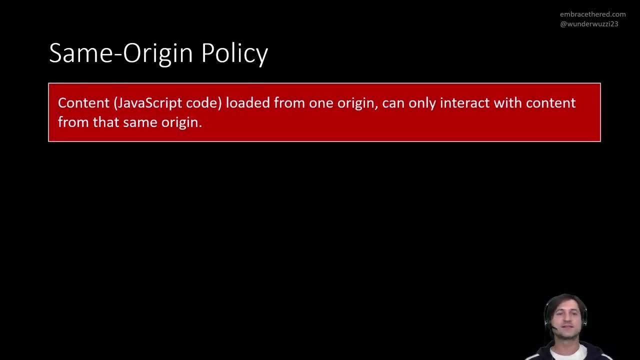 is sort of the same origin policy. So the same origin policy basically tells or is defined in a way that if you load content or JavaScript in particular from one specific origin, then that code or content can only interact with that particular origin. So maybe what's sort of a little bit confusing right now. 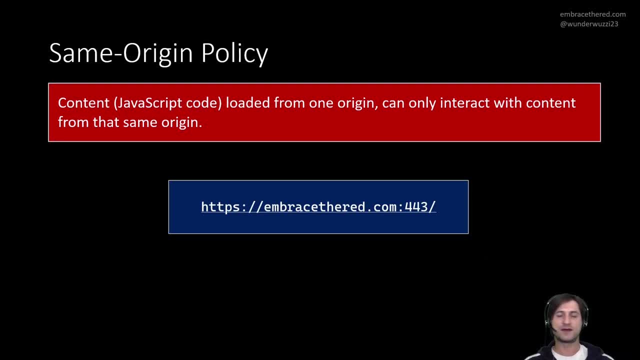 is what is actually an origin. So let's look at that first before we go into very detailed examples. So this is an origin. It consists of three parts, which is the protocol in the very beginning, or the scheme. It's called scheme, in this case HTTPS. 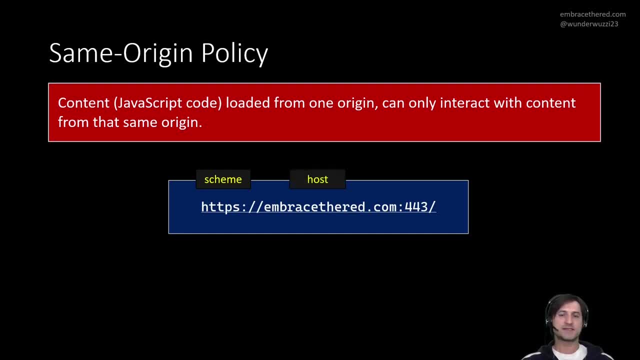 Then the host name, which in this case embraces the red, and then the port. So those three pieces together make up the origin. And now let's look at an example. So these are all different origins. We have exampleorg and exampleorg from port 8080. 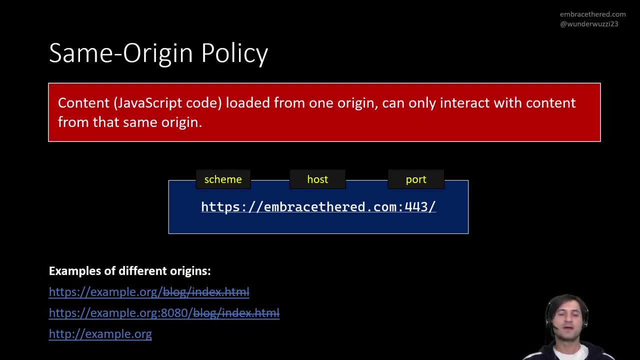 and then one that is HTTP exampleorg. So all of those three are different origins. I did like strike out the later part of the URL because that is not relevant when it comes to looking at the origin. So what the same origin policy now says? 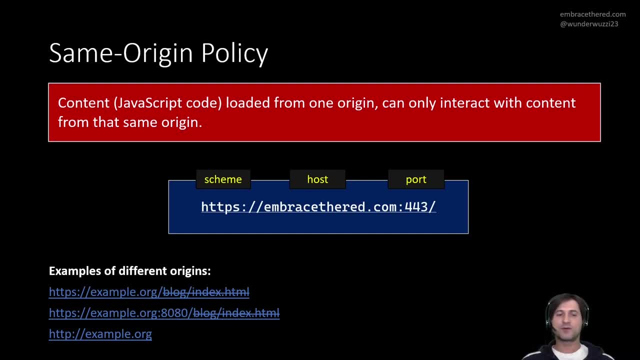 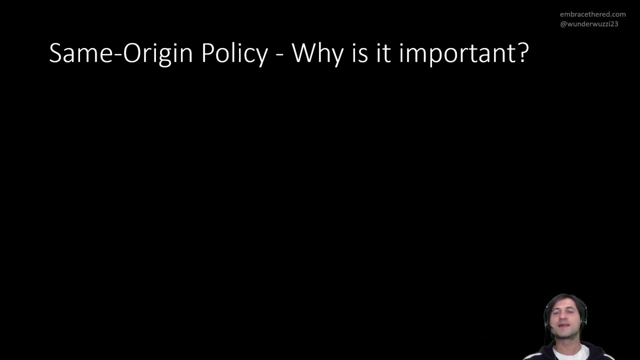 is that if JavaScript is loaded from exampleorg, it cannot access HTML from exampleorg on port 8080. So this is not possible. So yeah, the question is: why is this important? right And sort of. I already kind of said that. 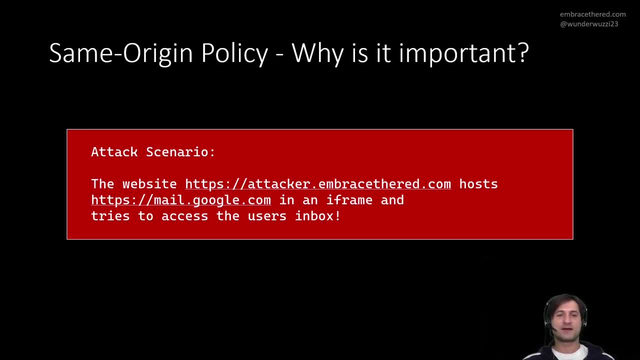 because in a worst-case scenario- consider this attack scenario- You have a website called attackerembracetheredcom And that website. you visit that website as a user. For some reason, you might have clicked a link or browsed Facebook and somehow you end up on this website. 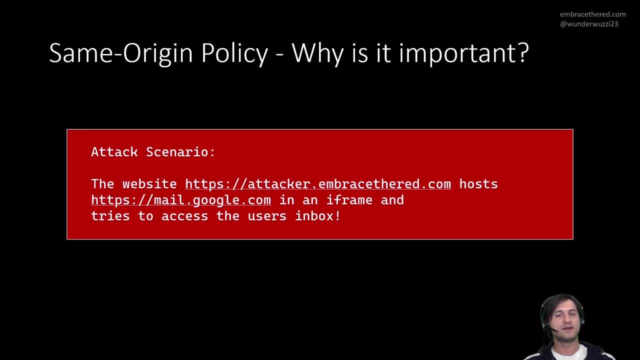 And that website loads Gmail into an iframe, which is an HTML tag that sort of allows you to embed another web page, And this would now mean that this attacker page can run code to access your inbox- technically right, And this is exactly what the same origin policy prevents. 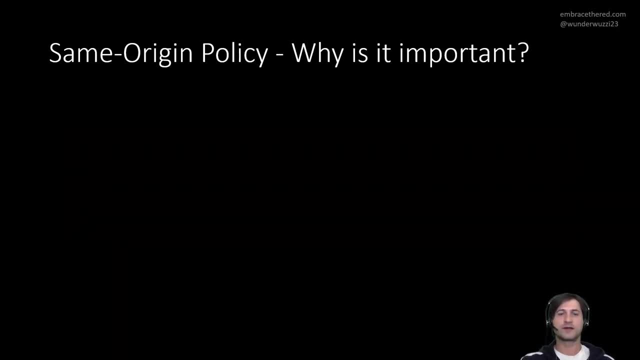 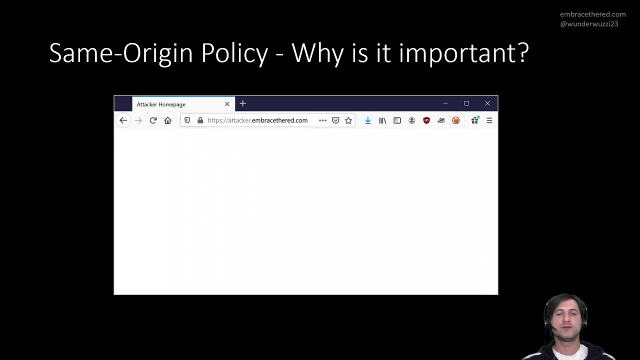 Let's look at an example. You know very kind of visualizing this concept. So this is the attacker homepage. You as a user, for some reason ended up on this page. So, and since it's attacker's page is, you know. 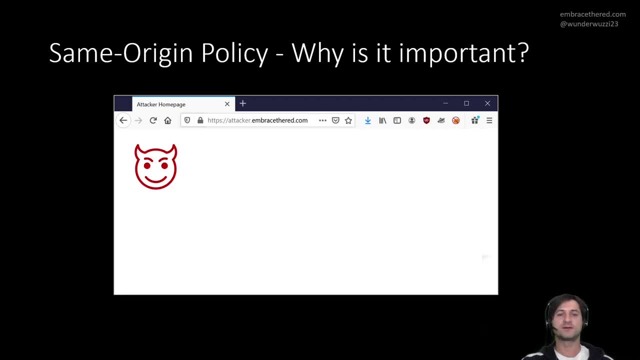 the attacker controls the code or the HTML document on it. And what the attacker did in this case? they created an iframe which points to Gmail, mailgooglecom, and loads your inbox or the inbox that you, yeah, your inbox- into that iframe and closes this. 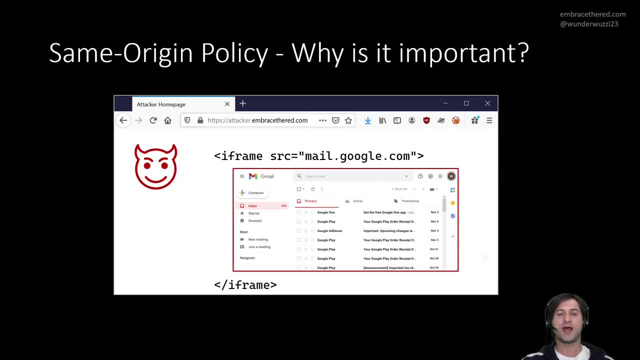 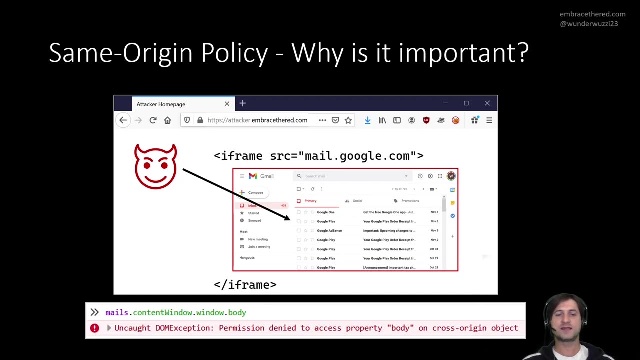 So now the attacker could try to access with JavaScript, right, He could now try to access this iframe and the content within that iframe. All right, And this is what the same origin policy prevents. So if you try this example and then you will see that JavaScript will give you this error, 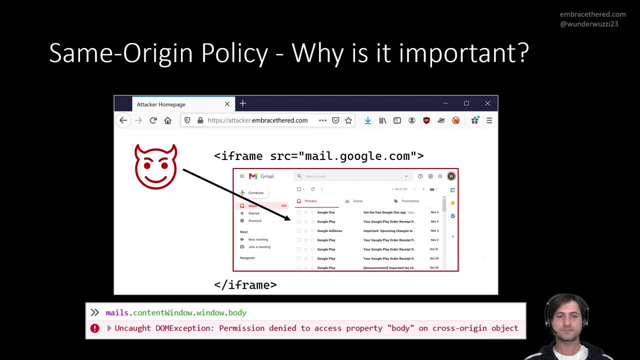 With a browser, the user agent gives you this error- It's an uncaught DOM exception- and then you get an access denied or a permission denied to access the body of this cross-origin object. So this is the same origin policy in action. 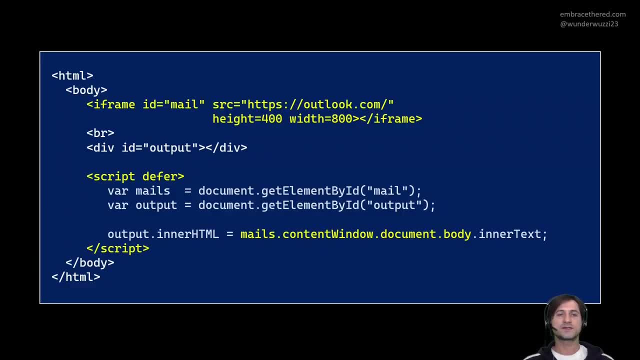 And to look at how this actually does look in code or in HTML, and code is. you can see here the HTML document. This is the attacker's website. It has an iframe with an identifier just called mail, And then it loads the source of you know. 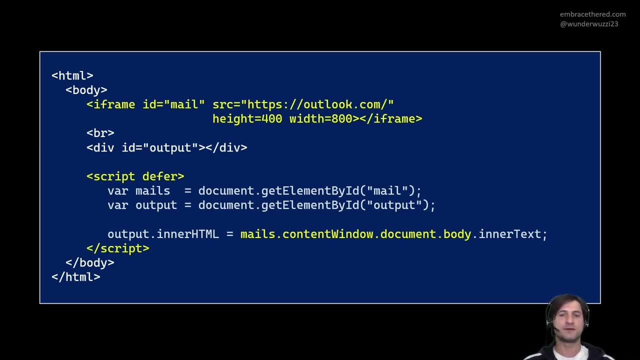 a web application like email program. In this case I used Outlook in the previous slide. Sorry, I had Gmail And so that loads this document. And then we have the script tag Defer just means don't run the script until it's done. 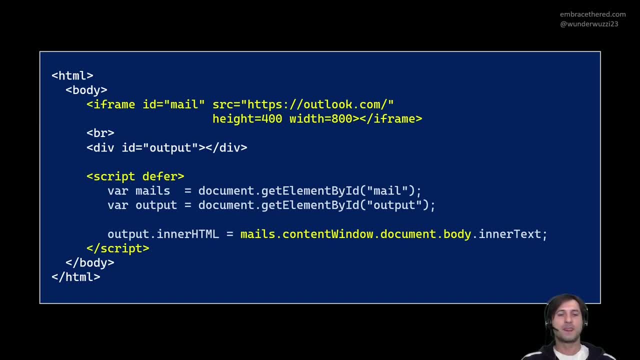 Don't run the script until the entire page is loaded. And this script particularly creates a reference. It does a document get element by the mail which is a reference to the iframe. Remember, the ID of the iframe is mail. And then we also get a reference to some place. 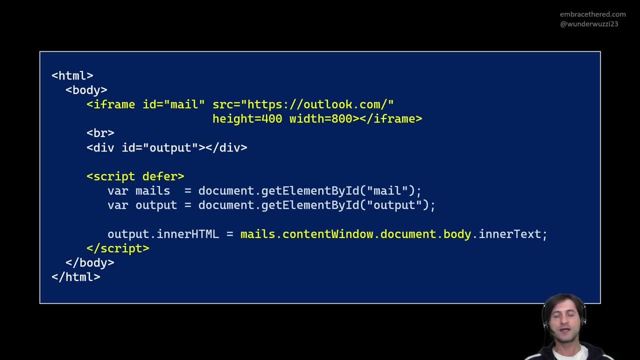 we can write the output to which is this diff. And the third line in the JavaScript is basically trying to access the mail content like the iframe and the emails in that iframe, And what you can see like this line here is sort of this line that tries to do the malicious thing. 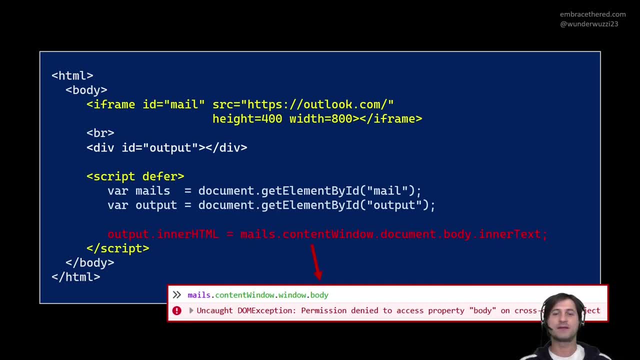 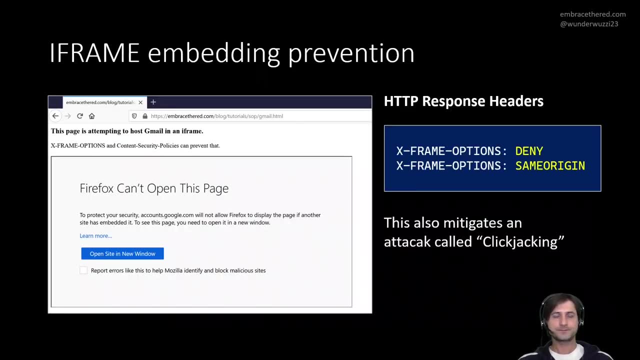 And when that actually happens, this is exactly when that permission denied occurs in the browser. So this is the same origin policy in action. If you actually go ahead and try this with, for instance, with Gmail, it's actually not, you won't even get as far. 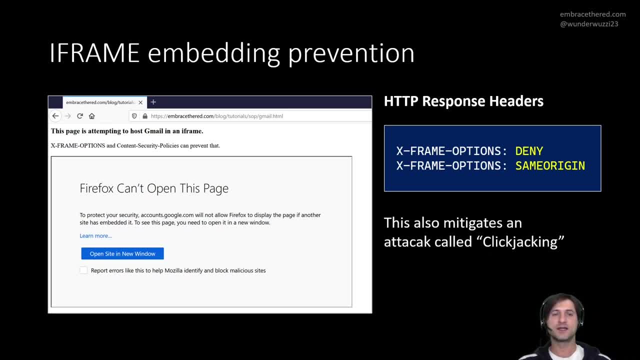 The reason for that is that there is an additional mitigation that was implemented by the web server, which uses what's called X frame options, which is sort of a mitigation to prevent framing or embedding one application in another. So if you have an application and you do not want, 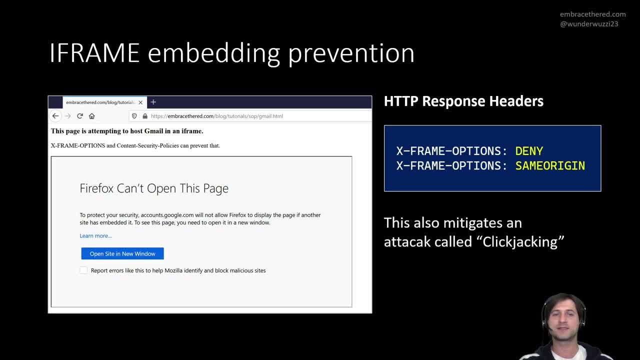 your own application to be framed or embedded by somebody else, by an attacker. you can set this HTTP response header X frame options, and then the browser will not allow a new application to be iframed. In this case, you see Firefox and you see the error message. 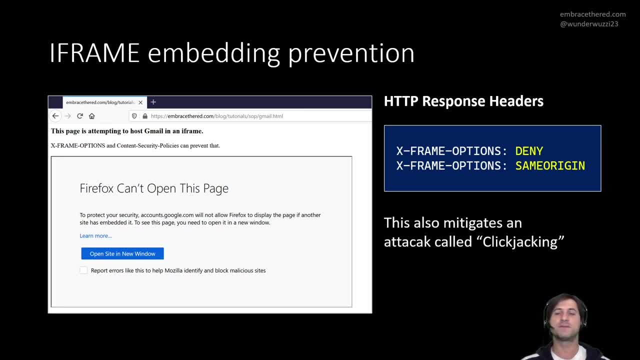 the security message that says you know this page cannot be put in an iframe. This actually has been implemented to mitigate an attack called click-checking. I'm sorry, I just saw it as a a slight misspelling. Yeah, so this was mitigated to implement click-checking. 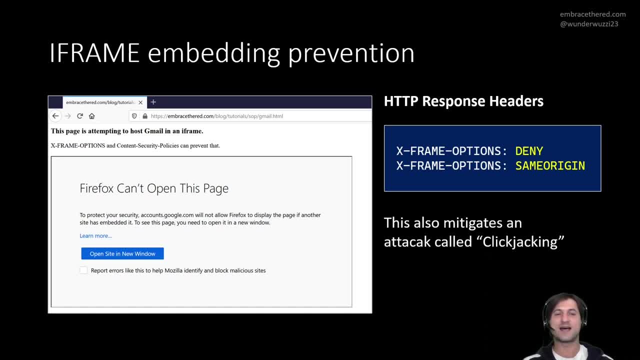 which is sort of a user tricking a user to click something that is not really visible at the moment by layering multiple iframes on top of each other. So you will click on one, but in reality you click on something that is behind it. 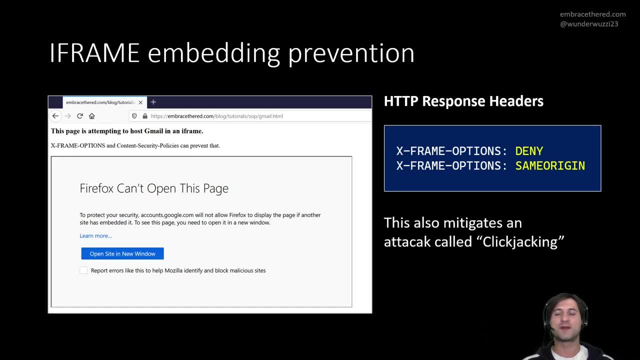 Let's say you know Amazon one-click shopping, You might overlay multiple iframes and then you click one button and in reality you click the checkout button. So this is click-checking, and X frame options sort of denies or prevents this by not allowing an attacker to frame. 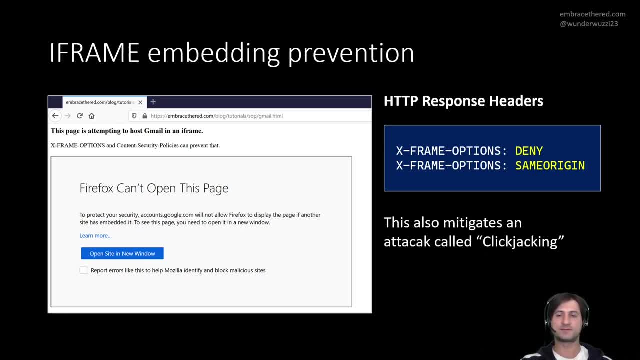 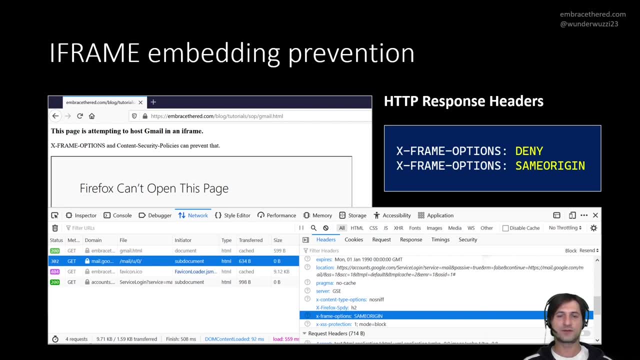 or embed another, the other application. If you look in more detail, you can actually also inspect this and I'm going to show you later how you can do this. but right-clicking and looking at the network traffic, you can see that the response here that comes back from Google. 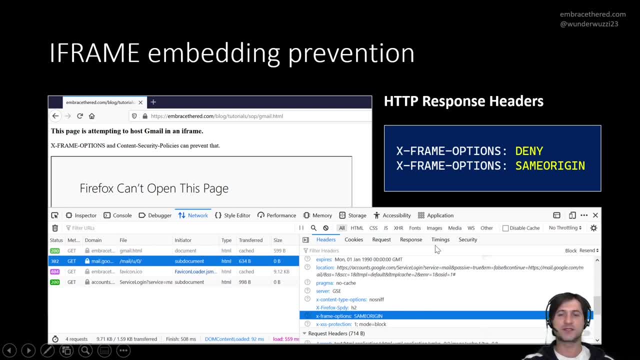 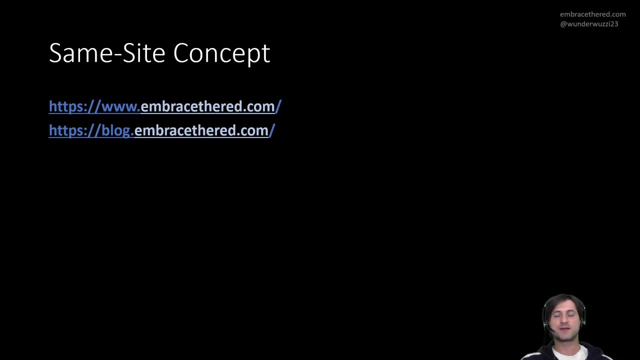 saying X frame options, same origin, and that's sort of how they implemented Gmail: to prevent being iframed. The next thing I want to briefly talk about, because this is becoming more important: this didn't exist a couple of years ago. 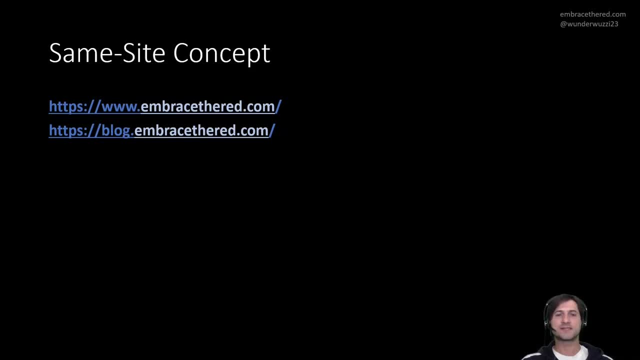 but now it becomes more important is this idea of same site. So same site means that you have this top-level domain that is sort of the same like Embrace the Red, and so the top-level domain plus one, so embracetheredcom. 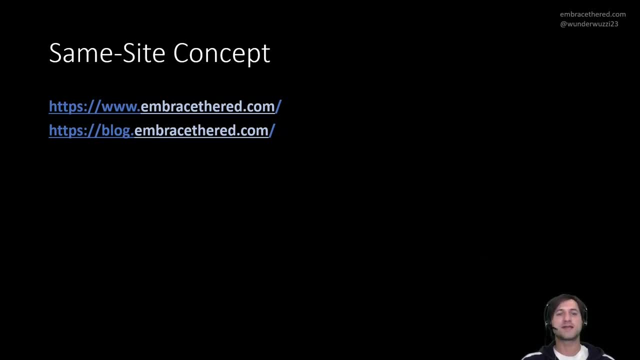 wwwembracetheredcom is same site as blockembracetheredcom, And there's a few kind of variations of that that are defined in this public suffix list, where you would have, for instance, things like GitHub, IO or so on. 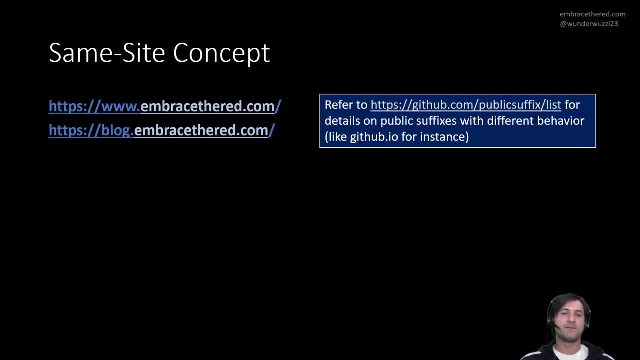 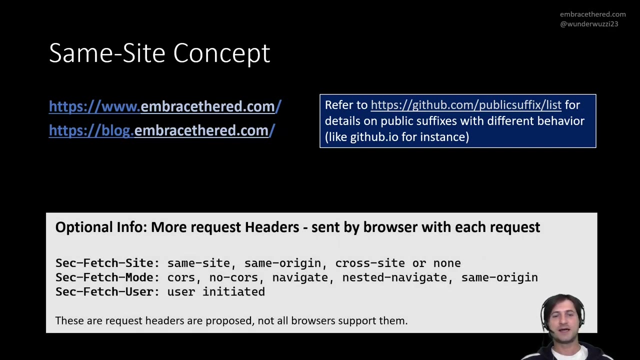 They have one extension to that, But it's not too important right now to understand the details, but just this idea of same site, that that concept exists. That's one thing that I want you to know, And along the same lines, there's more optional information as well. 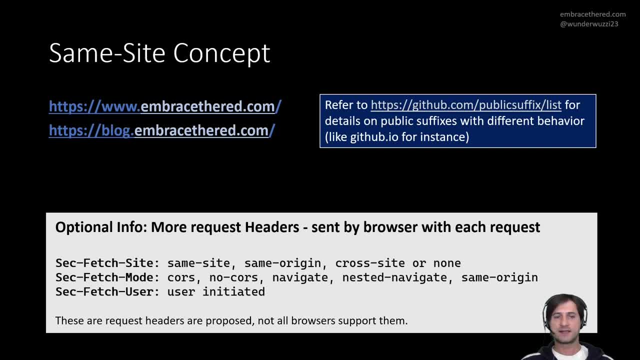 There's more request headers a browser sends And there's actually a lot of changes happening right now to browsers as well, where they tell the web server more information of where they came from And none of them are fully. they're not really implemented in all the browsers. 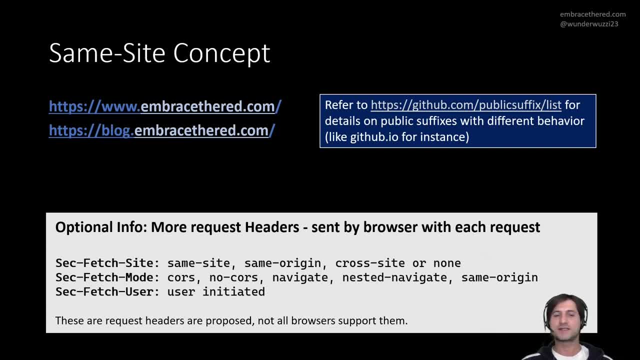 but I kind of want you to be aware that this change is going to happen And I can do a session about those three HTTP headers in particular. if there's interest, So just mention it in the comments and I'll dive into the details of those three. 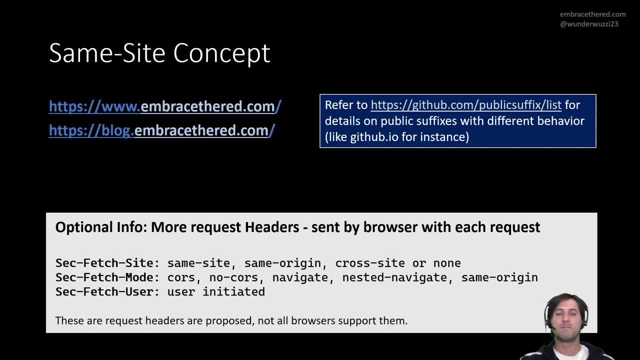 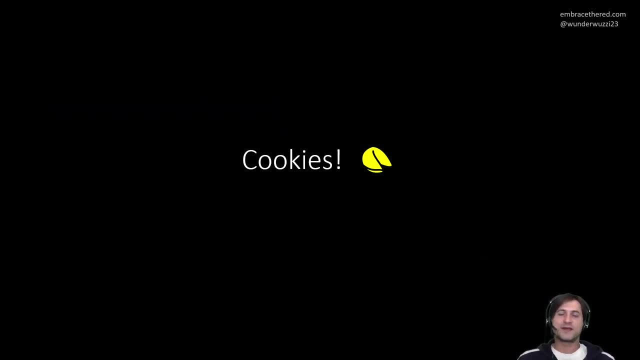 Because they allow preventing a lot of attacks actually in a very simple way or have basic mitigations for some of the web replication attacks And it can be implemented simply on the server side. But the most important thing that I want to talk about in this entire kind of session, 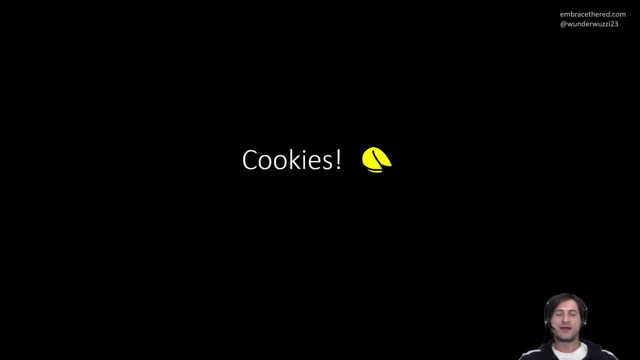 about the web replication. security fundamentals is cookies, Because a lot of security web replication revolves around cookies. So what is the cookie? So imagine again our web replication, which you see on the left, and our web server that is on the right. So we said, you know we click a link. 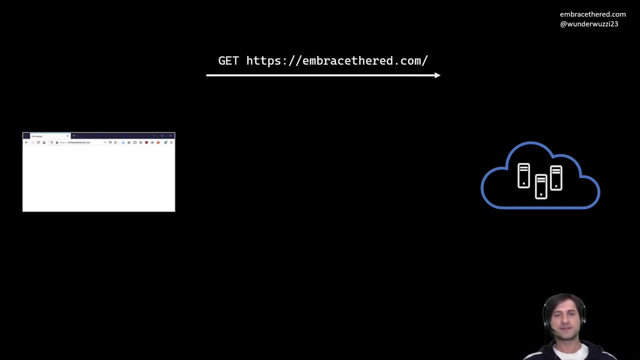 we visit the web page and the browser issues this GET request, The server now renders this page right, creates this HTML document and, in our case, now also creates a cookie And sends both of these pieces back to the user, to the client in the user agent. 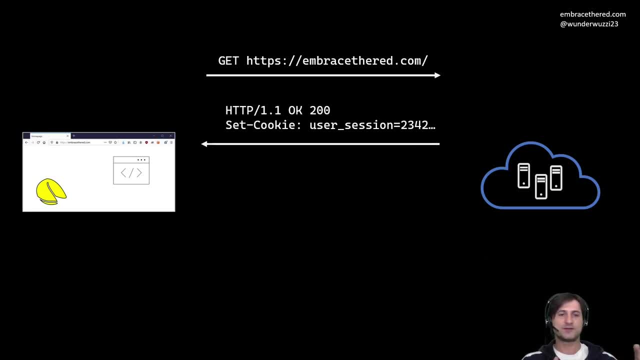 So the user agent now has the web application- you know this HTML document- and it also has this cookie. So what is a cookie now? So a cookie now, and I put a safe here because the browser kind of needs to kind of store the cookie very securely. 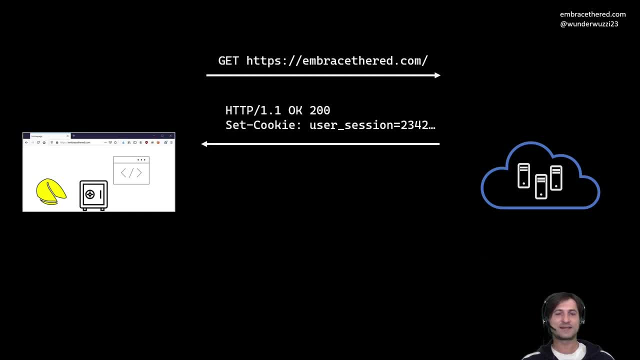 and hold it very safely, And you will understand in kind of just a few moments why that is So. now, every single time the browser visits the web server, embraces the red again, it will send that cookie back to the user agent, To the web server. 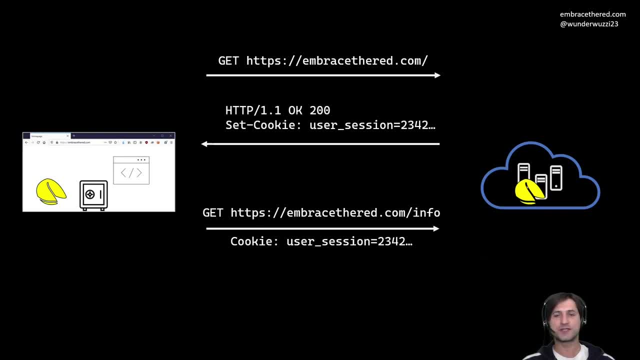 So just the fact that the domain matches this origin matches, the cookie is being sent back. Actually, the site matches. That's why the cookie is being sent back for this request. So any cookie that a browser stores for a particular domain will be sent automatically. 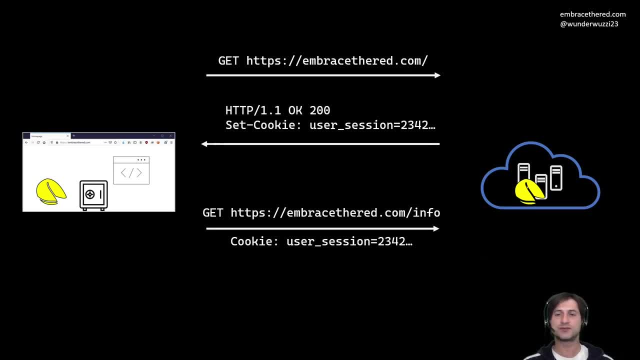 So there's nothing. the code, JavaScript or anything needs to do Anything, any click and this cookie is being sent. So this was the first click. visiting the info page, There might be a post to an update endpoint Again when that post happens. 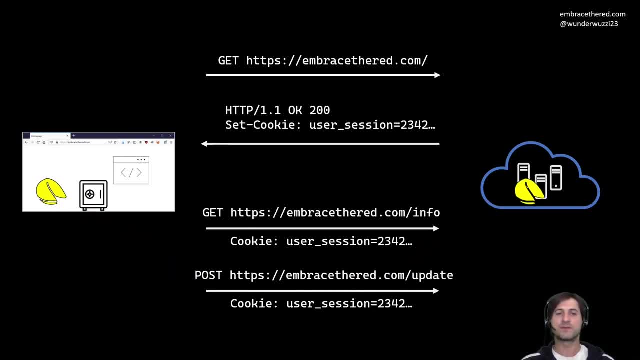 the cookie is being sent with the request to the server. So the reason this was implemented is because HTTP is stateless And this means there's no- it's kind of difficult to create a session- this idea of a user being authenticated. So that is this one way. 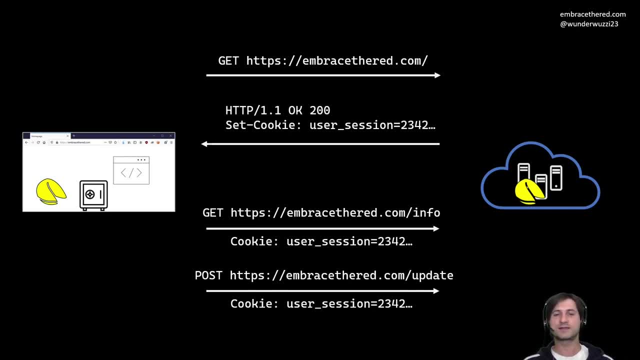 the HTTP specification allows to create sort of a session concept, which is the cookie, which is a piece of data stored in the browser, And whenever the user visits a particular domain again for which the browser stores a cookie, the cookie will be sent by the browser. 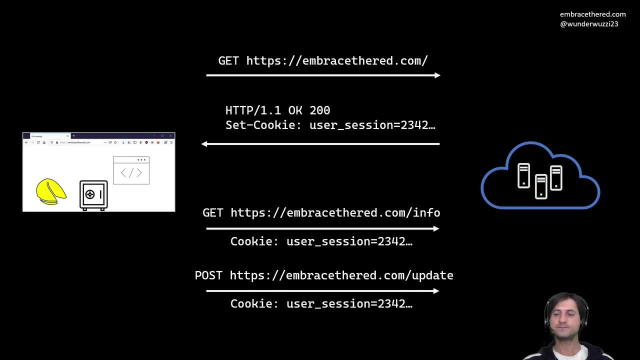 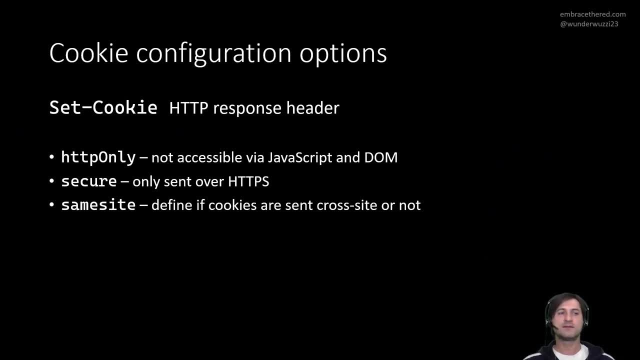 to that web server. So, as you can see, the cookie is very important because if somebody steals that cookie, they can impersonate somebody else, So they can impersonate that session. In order to prevent that, there are actually a couple of mitigations. 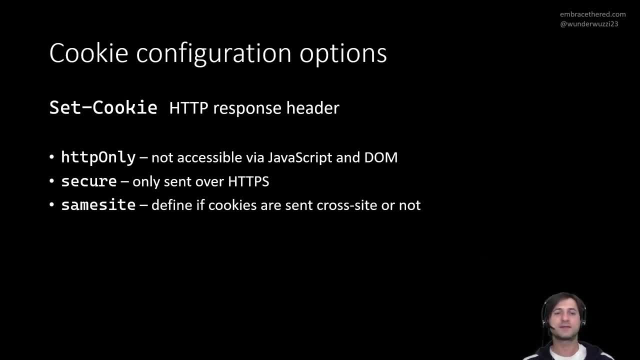 that can be set as part of an HTTP response. when setting the cookie, with the setCookieHttpResponse header There's HTTP only, which sort of defines that the cookie is not accessible from code, from the JavaScript. So it is only in transport. So HTTP only, only in transport. 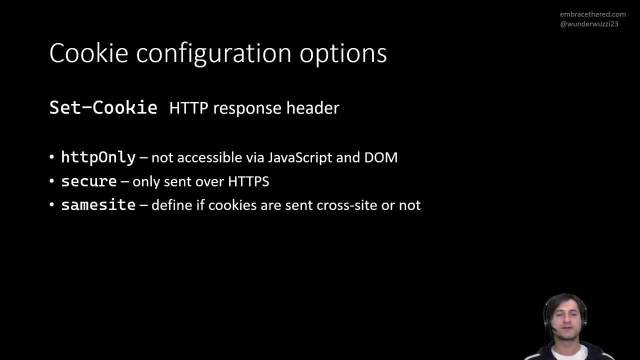 So it sort of becomes invisible to JavaScript. The second mitigation is applying something that is called secure, which is basically a setting that says the cookie will only be sent over an HTTPS connection, which is an encrypted connection. So it will not be sent if the connection is not encrypted. 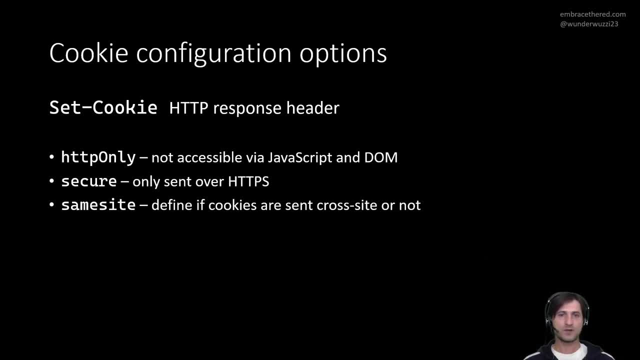 So if there's somebody in the man in the middle or maybe in a coffee shop or something, somebody might sniff the traffic and gain access to the cookie. if it's not sent over HTTPS, this secure attribute or flag will prevent that. So very important when setCookie happens. 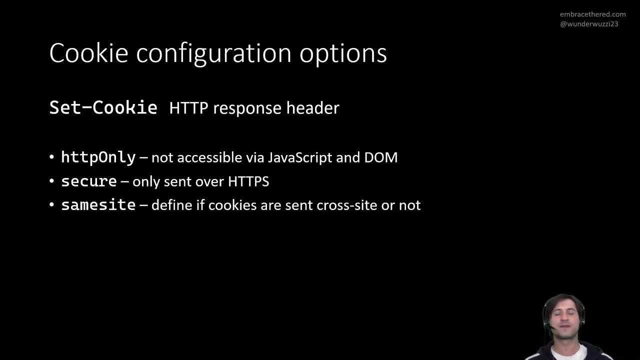 from the web server initially to set the cookie, for the client to specify the secure flag. The third flag is same site, which is actually pretty new, But this specifies if the cookie is sent across site or not, which is sort of also a little bit of a mitigation. 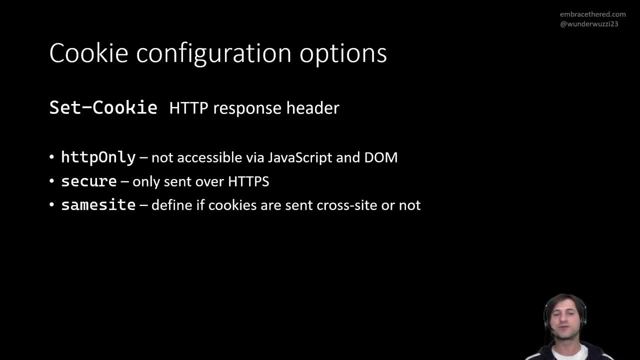 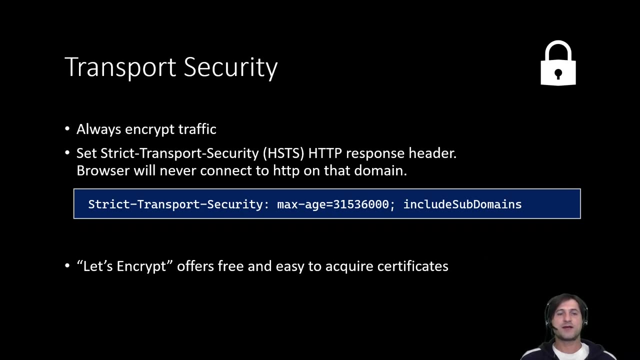 for advertisement tracking. right, Because cookies are used for by companies like Facebook and Google to track you across the internet. right, Because that's sort of what these cookies allow. A little bit more about transport security I just wanted to bring up here is that. 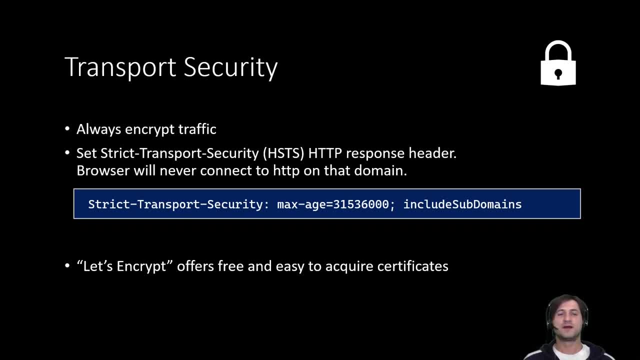 you know, traffic should always be encrypted, So there's really no reason anymore to not have traffic encrypted. This actually is even true for internal applications, Like if you have an internet, all your traffic should be encrypted. There's also this HTTP header- response header. 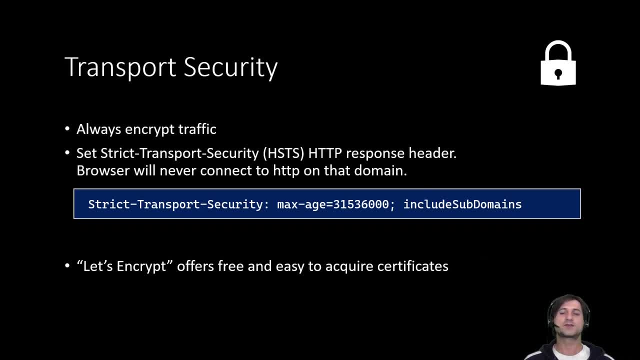 called strict transport security, which sort of instructs the browser to always upgrade to HTTPS. So even if there's like a, you have a spelling mistake in one of your links or URLs and you type HTTP instead of HTTPS, the browser will automatically replace that with HTTPS. 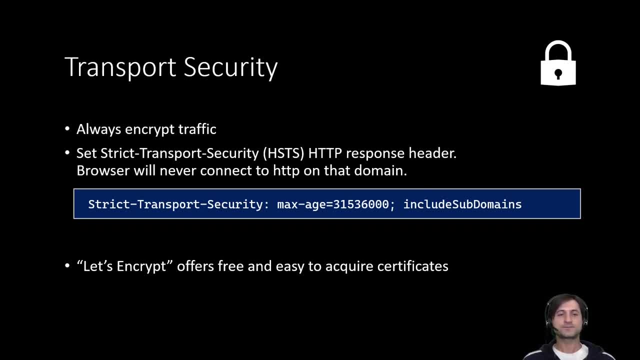 So this is strict transport security And if you kind of worried on having to pay a lot of money to get certificates, look into Let's Encrypt. I'm using this for my own websites. It's very easy to use, It's free. 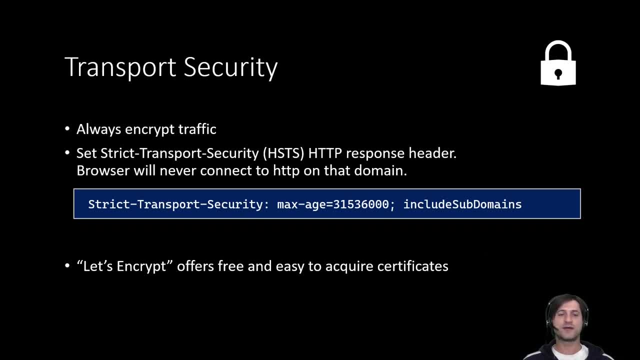 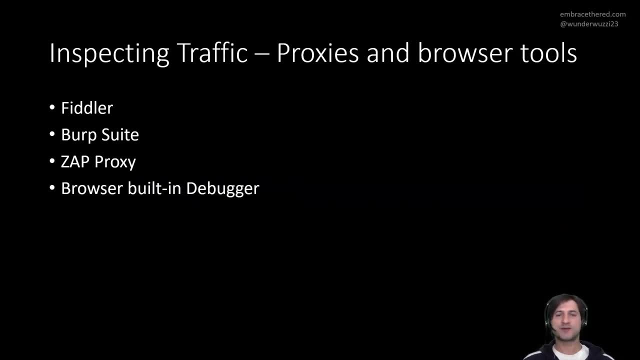 And there's a good way for you to get valid certificates. Speaking more about- actually you know, inspecting traffic, looking at HTML documents and proxying requests, There's a couple of tools I've been using throughout my kind of security endeavors. 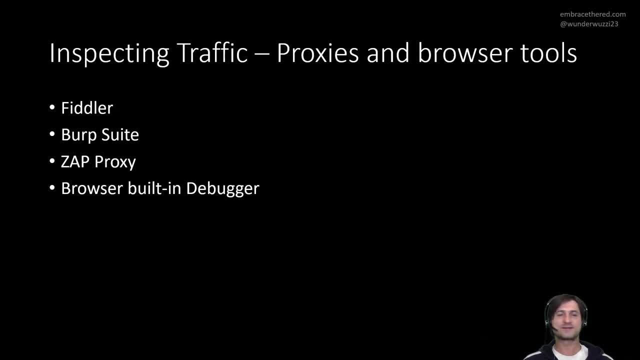 On Windows. I really like Fiddler, which is free and it just plugs in nicely into the browser And it's very simple to use. Then there's Burp, there's Zap and also the browser has. browsers have built-in debuggers. 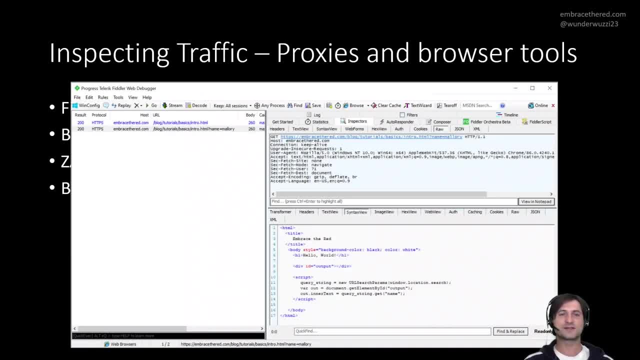 that are really useful. So let me just quickly show you Fiddler real quick. So this is Fiddler in action and it's turned on. You open it on the left and you see all these requests that the browser issues, And on the right 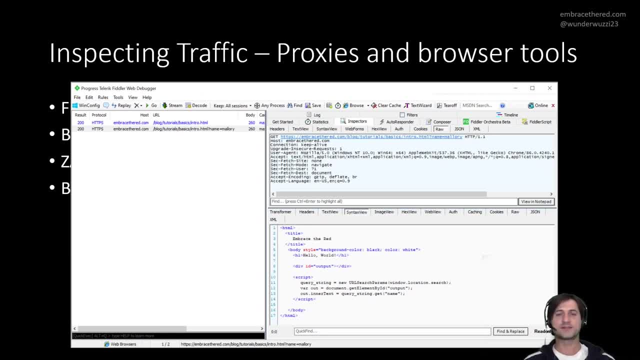 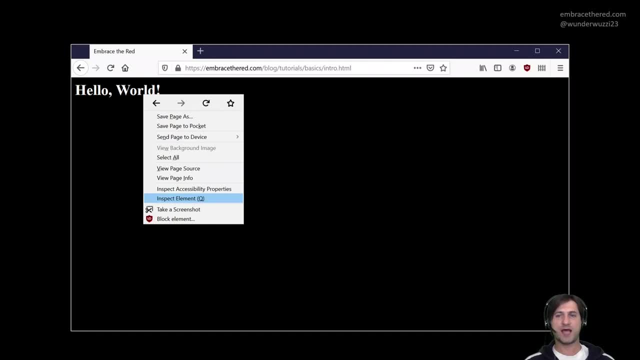 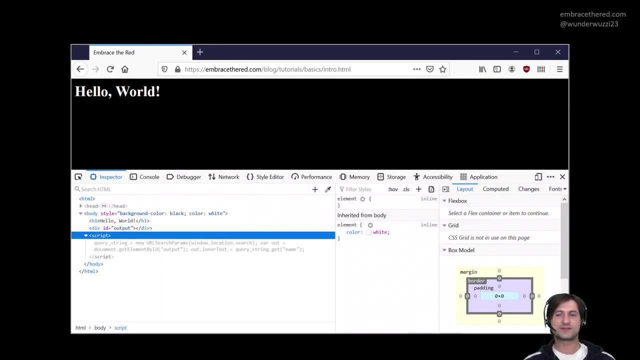 you see the details of the request and the response nicely shown in the UI. Similar. if you just have the browser, you can right-click anywhere in the document and do inspect element. That takes you then to this web developer view where you can see here on the left. 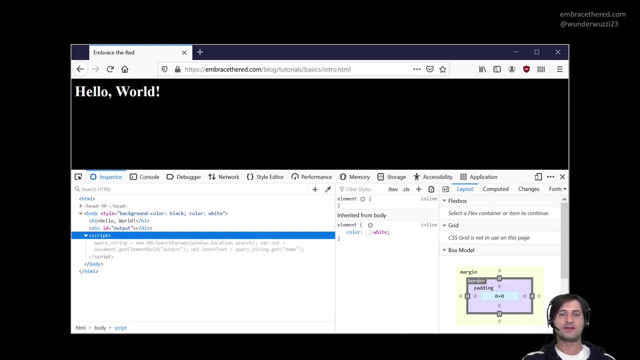 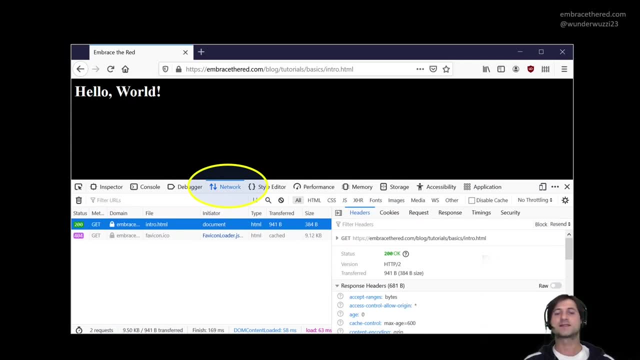 you see the actual HTML document and you can also click on this network button up here and then takes you to the view of seeing the HTTP requests and responses. So this is actually super useful and this is every browser nowadays actually has these web developer tools built-in. 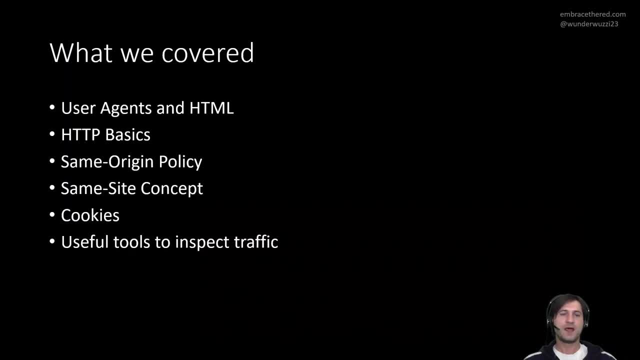 It's super, super convenient. Okay, so this sort of wraps up this very first session. It was a little bit basic and I hope I was able to convey sort of these foundations which will allow you to understand all the attacks that we're going to talk. 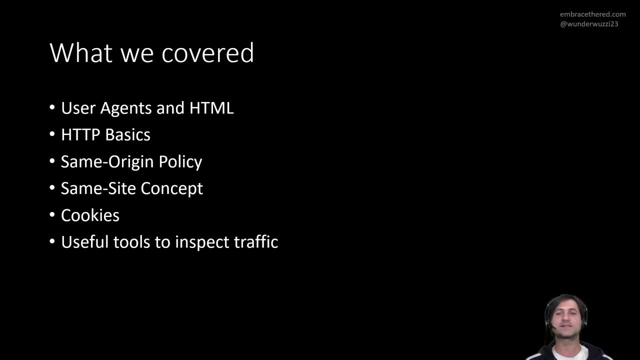 in the next couple of sessions pretty easily, I think. Again, we learned about user agents, we learned about HTML, about the transport protocol of HTML. we learned about the same origin policy, the same site concept. We talked a lot about cookies. 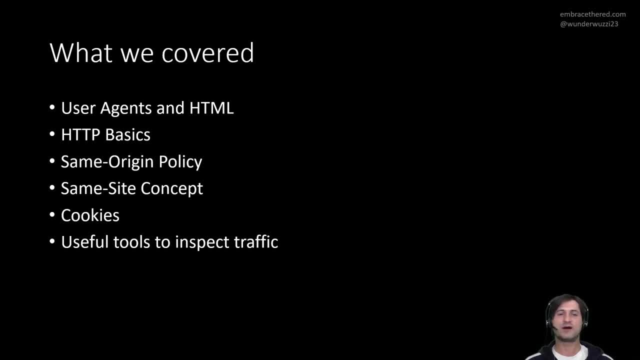 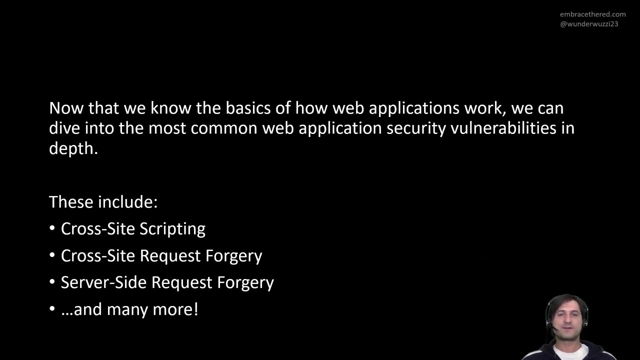 and that HTTP is a stateless protocol and cookies sort of can help you get state and kind of create sessions across multiple requests, And in the end we looked at a couple useful tools. So, yeah, that's sort of wrapping it up now. 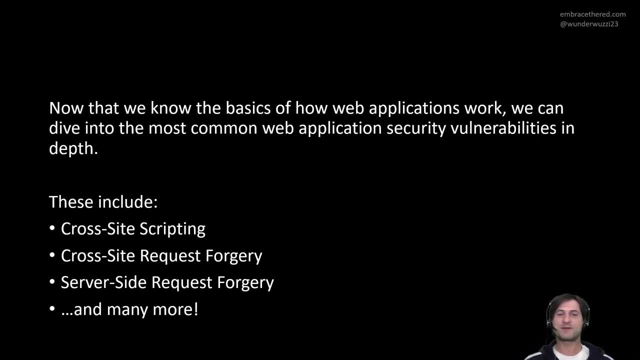 There will be more videos coming up. I'm going to talk about cross-site scripting, tab nabbing, cross-site request, forgery, many, many more. If there's any sort of particular attack you want me to go into detail, let me know. add a comment. 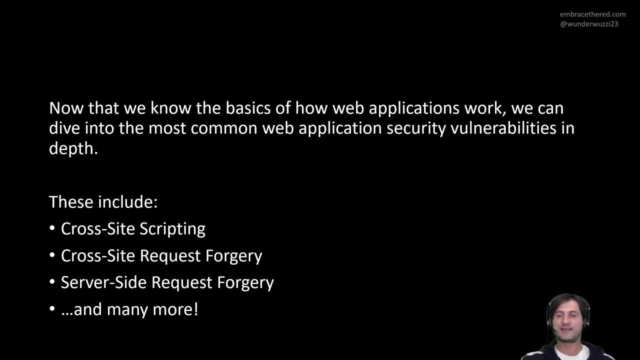 and I'll create a video for it. Thank you so much for watching. I hope this is useful. Make sure to subscribe so you get notifications when I post a new video. And yeah, have an awesome day.